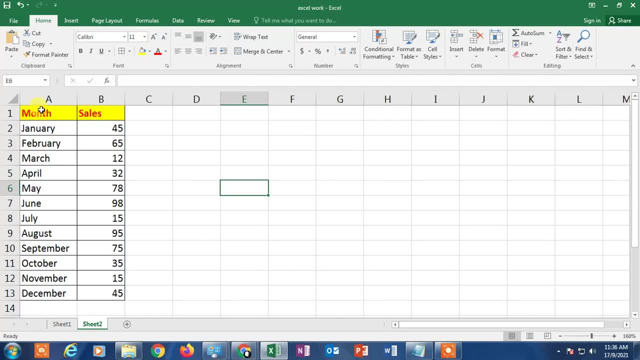 So here I have Excel and this is my demo data, like sample data I have just created, like month wise and month wise sales. So I want to apply the color scale in this table to spot maximum and minimum values. okay, by color, okay. So, guys, in order to how to use color scale in Excel, just create your data and select the data range you want to use. 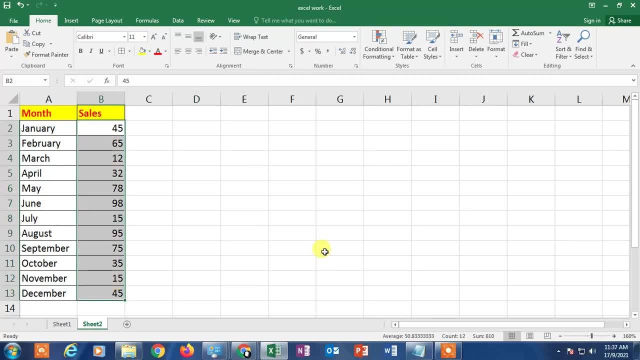 So I want to apply color scale, okay, and here you have to go in home and now you have to click on conditional formatting. This will applied with using condition formatting. Click on this and here you can see the color scale and you can see the. there is a many format sample that you can apply it. So if I apply this one, you can see the minimum value is red and maximum value is green. Okay, so you can find out the. 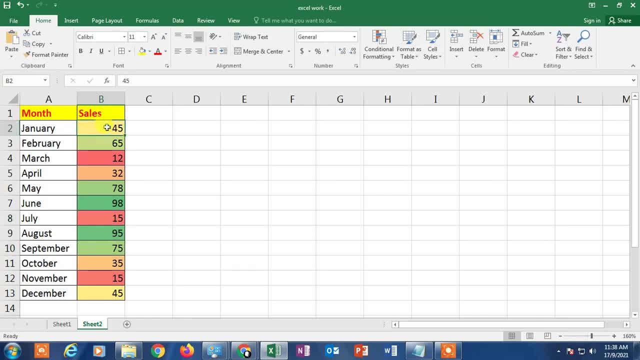 which one the maximum value and which is the minimum value. So here you can see: minimum value is 15 and maximum value is 95.. Okay, so if you want to edit color scale or if you want to add three color or four color in the color scale, you can add this. So here, select any cell where you use color scale. Now you have to click on conditional formatting here and click on. 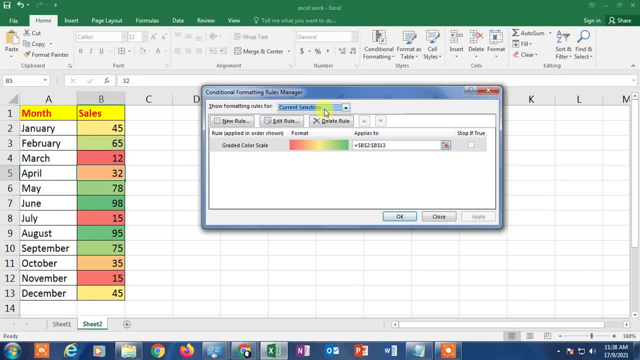 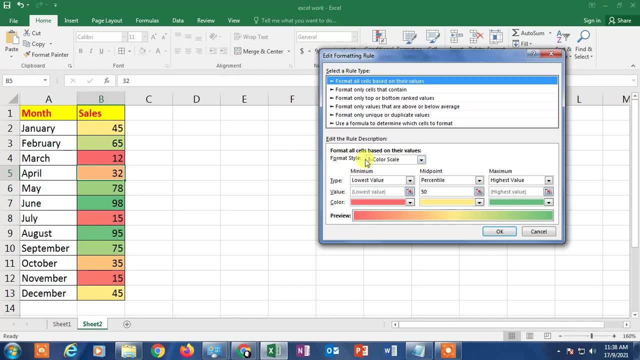 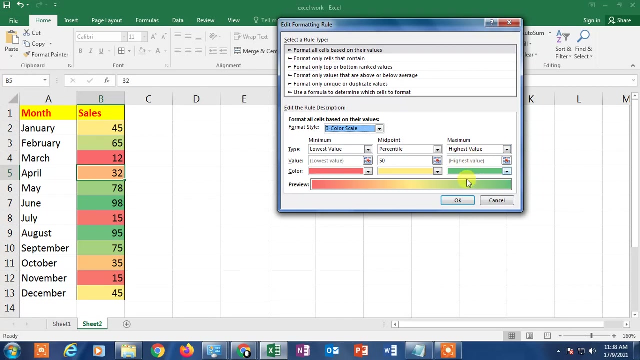 manage rules. In manage rules you can see current selection. Okay, edit rules. click on the edit rules and here you can see you can select color from here, like three color, two color. So we have option with three color and two color. Okay, so if you want three color, you can keep it. Now you can see lowest value and highest value colors. Okay, so you can change color from here like lowest value color. you can if you want to change. 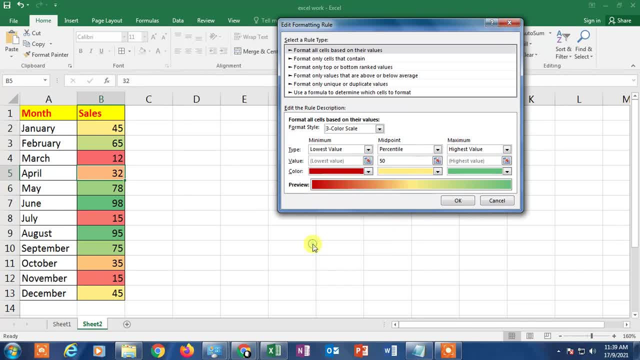 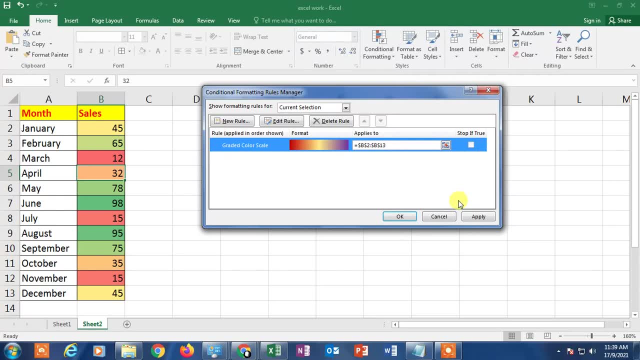 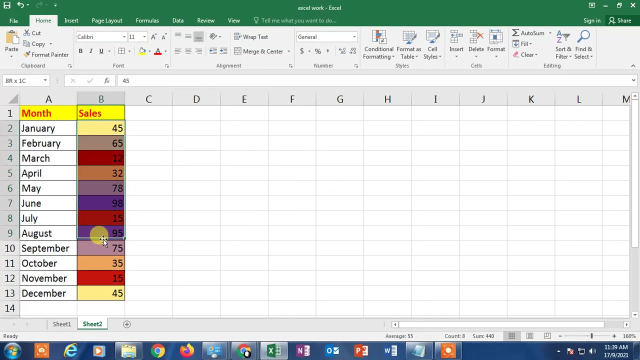 to give the dark red and highest value. you want to give this one. okay, so click on this and now apply so you can see color has been applied now. okay, so now, if you want to clear colors, color scale from your table, just click the alt table or you.